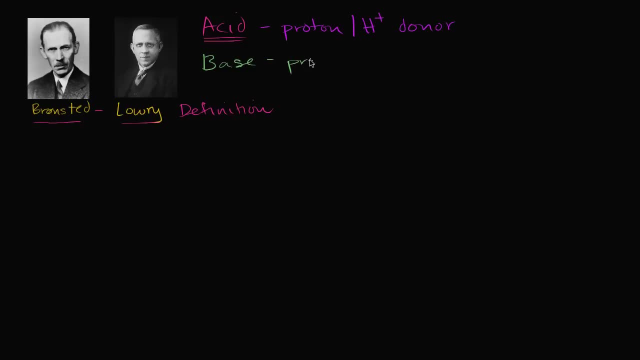 a base would be a proton or you could say a hydrogen ion acceptor. So let's make this a little bit more tangible with some examples. So one of the stronger acids we know is hydrochloric acid, And let me draw. So it's a hydrogen having a covalent bond. 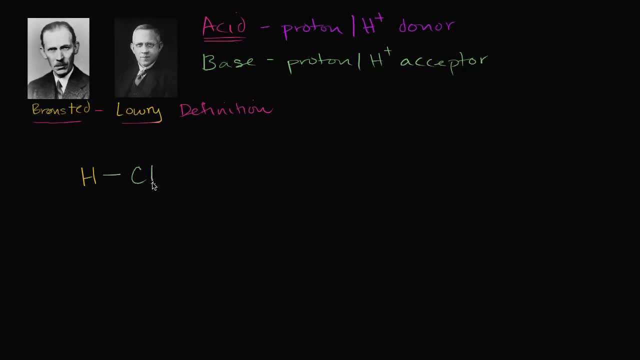 with chlorine right over there And if we want to, let's draw actually chlorine's lone pair. So outside of the electron that is contributing to this pair in the covalent bond, it also has three other lone pairs. It also has three other lone pairs. 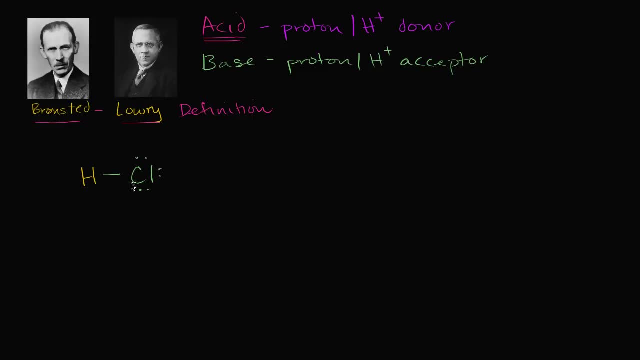 Just like that. So if you were to take hydrochloric acid, place it in an aqueous solution. So it's in an aqueous solution right over here And actually an aqueous solution. you'll see this written like that. 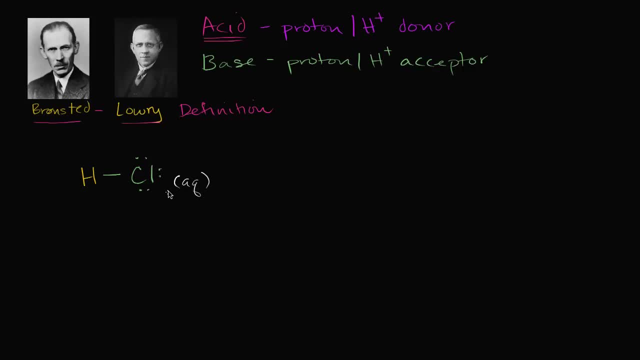 That just means it's in a solution of water. So you could write like this. You could write hey, hydrochloric acid in an aqueous solution. If you want to make it a little bit more explicit, you could say: hey, look. 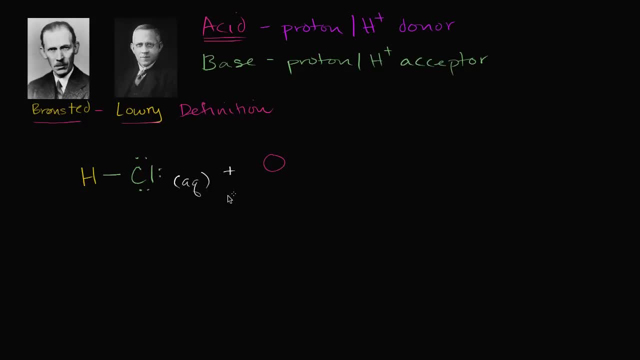 this is going to be around- some water molecules in its liquid form. Aqueous solution means it's dissolved in liquid water. So some water molecules in their liquid form. So this is a water molecule right over here. So an oxygen bonded to two hydrogens. 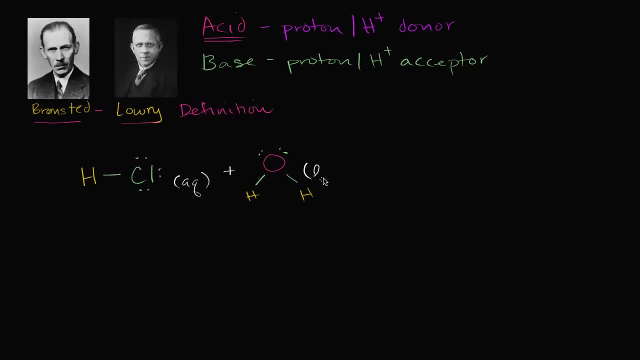 And sometimes you'll see it written like this, that it's in its liquid form. Well, what do you think is going to happen? Well, I already said that this is a strong acid right over here, So this is going to really want to donate protons. 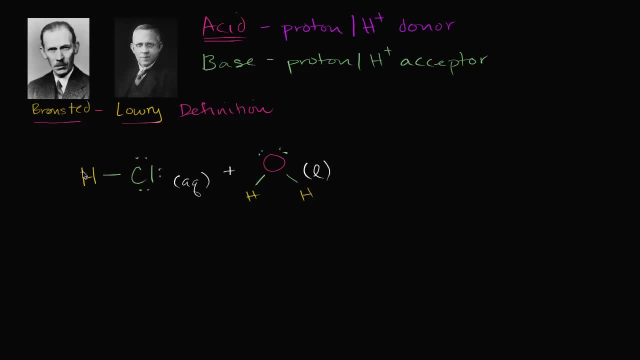 It's really going to want to donate this hydrogen, but not let the hydrogen keep its electrons. So what's likely to happen here? Well, both of these electrons in this pair are going to be grabbed by this chlorine And then this hydrogen ion. 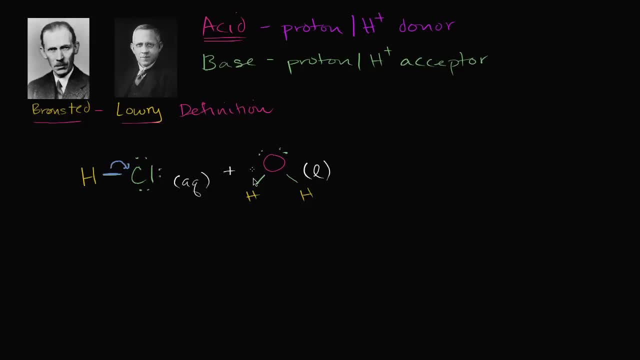 because its electron was grabbed. well, this could be nabbed by some water molecule passing by. Remember, in a real solution, it's not like they know what to do, They're just all bumping past each other And based on how badly they want to do things. 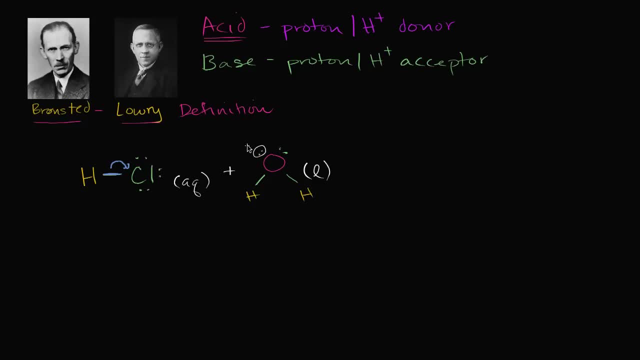 these reactions happen, And so you can imagine this lone pair right over here. well, maybe it's able to form a covalent bond with this hydrogen, And so what's going to happen- And I'll draw it with just an arrow because this reaction favorably goes- 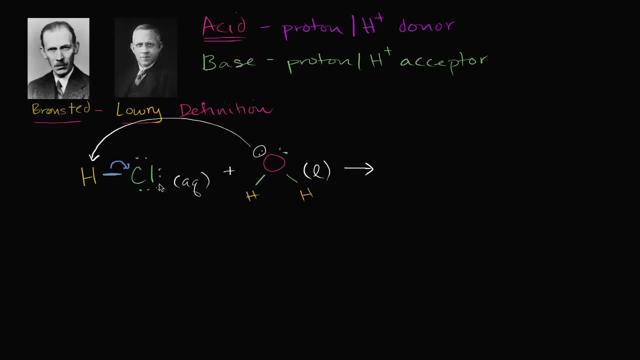 very strongly goes to the right because this is such a strong acid. Well then, you're going to be left with. you're going to be left with your. chlorine is now going to have its three lone pairs that it had before, And then it also grabbed these two electrons right over here. 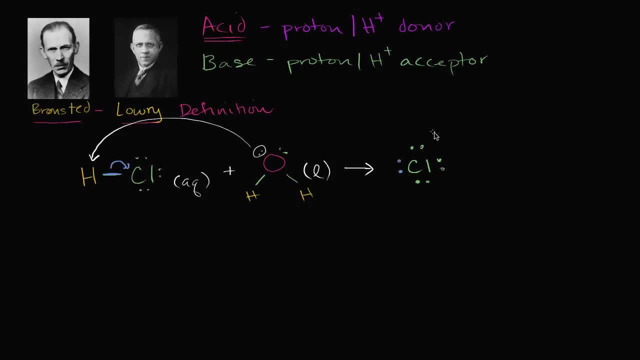 It also grabbed those two electrons right over there, So it gained an extra electron. It now has a negative charge. It is now the chloride anion, So it has a negative charge. And what about this water molecule? Well, this water molecule. 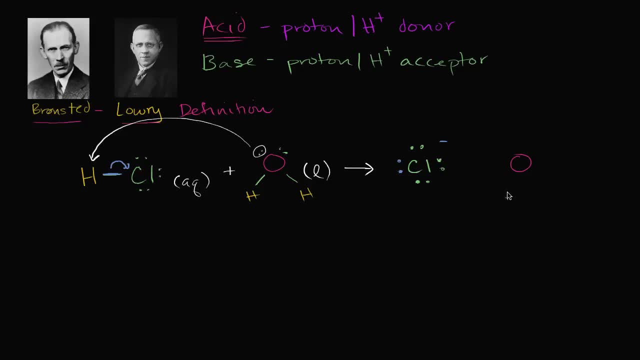 you have your oxygen, you have your hydrogens, you have your hydrogens, But now you don't just have two hydrogens. You grabbed this hydrogen right over here. Maybe I'll do this hydrogen in a slightly different color so that you could keep track of it. 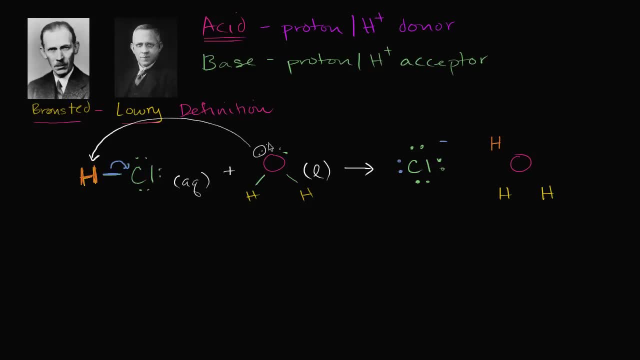 You have this hydrogen right over there And this lone pair, this lone pair you can view it as now forming this covalent bond. You had your other two covalent bonds to the other two hydrogens And then you still have this lone pair right over here. 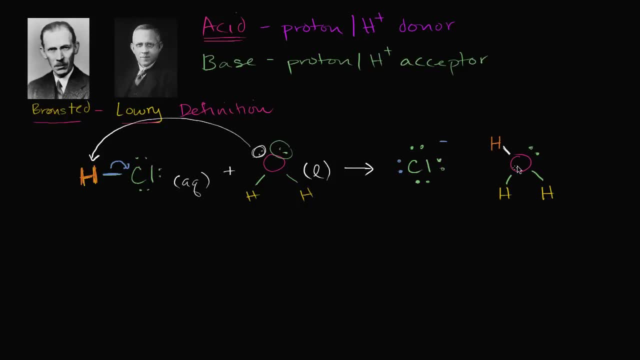 You still have that lone pair sitting right over there. And what just happened? Well, this water molecule just gained a proton. This hydrogen did not come with an electron. So if you just gain a proton, if you were neutral before, you are now going to have a positive charge. 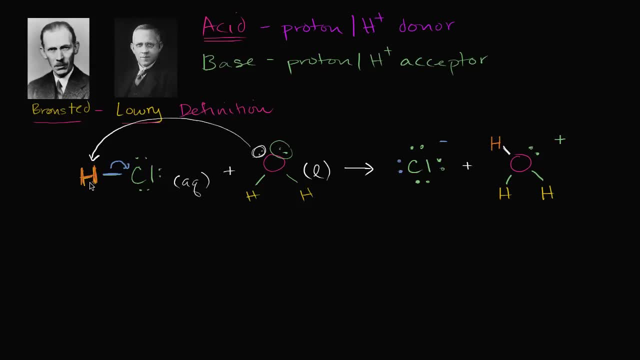 So what just happened? You put hydrochloric acid in a water solution. in an aqueous solution, This thing has donated a proton to a water molecule. And so what is the acid and what is the base here? Well, when we look at the reaction this way: 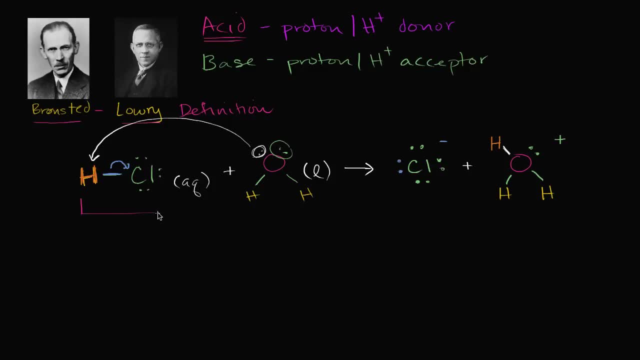 we see that this is the acid, the hydrochloric acid. It's literally called hydrochloric acid, And here water is acting as a base. Water is acting as a base And, as you can see, water can actually act as an acid or a base. 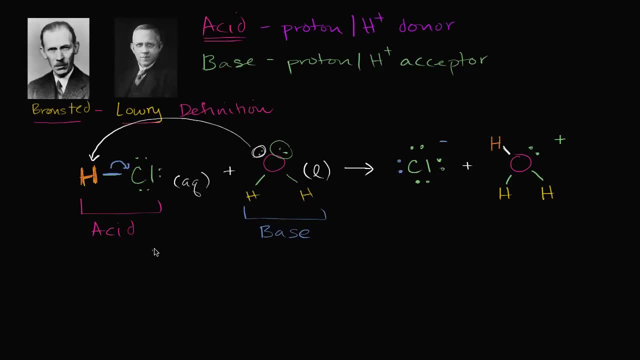 So water is acting as a base. Now you might be saying, okay, this reaction goes strongly to the right, Hey. but like you know, I could imagine there are certain circumstances where chloride might accept a proton because it has this negative charge. 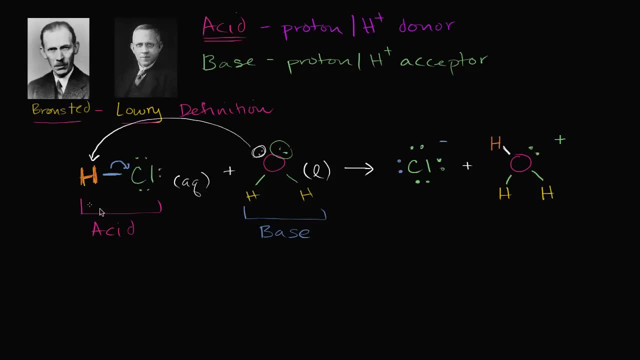 And you would be right. This reaction goes strongly to the right. But once an acid has donated its proton, the thing that is left over- this is called a conjugate base, And I'll do it in the same color. So this is the conjugate base of hydrochloric acid. 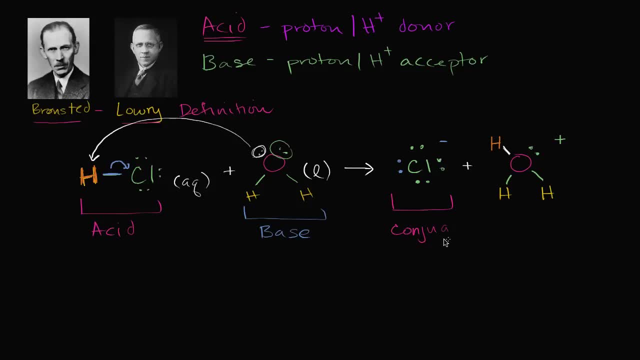 the chloride anion Conjugate base of hydrochloric acid, And this right over here is the conjugate acid, Because you could imagine this hydronium ion. this could, under the right circumstances, donate protons to other things. 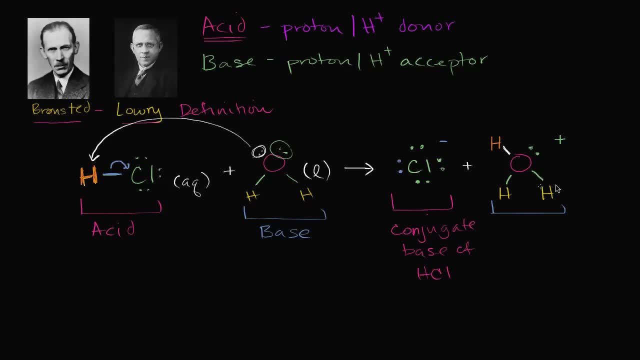 donate hydrogen without donating electron to other things, And so this is actually a conjugate, the conjugate acid of H2O, Conjugate acid of water, of a water molecule, And, as we'll see, water can act as an acid or a base. 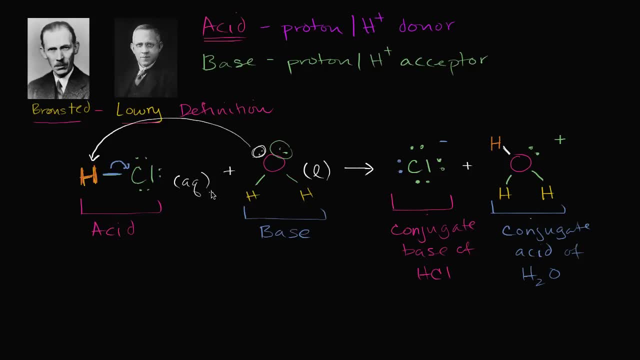 But this gives you a kind of a baseline of at least the Bronsted-Lowry definition of acids and bases. And actually one other thing I want to add In some books here. so over here I said, hey, you put this in an aqueous solution. 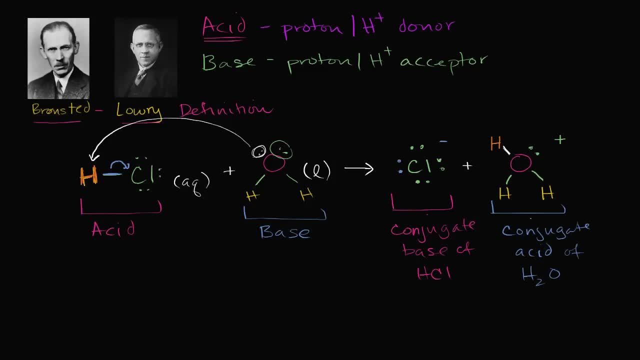 you're going to form some hydronium. Sometimes you'll see it written like this, And I'll just write it a little bit. Sometimes you'll see it like this: So you have your hydrochloric acid, and I won't draw all the details this time. 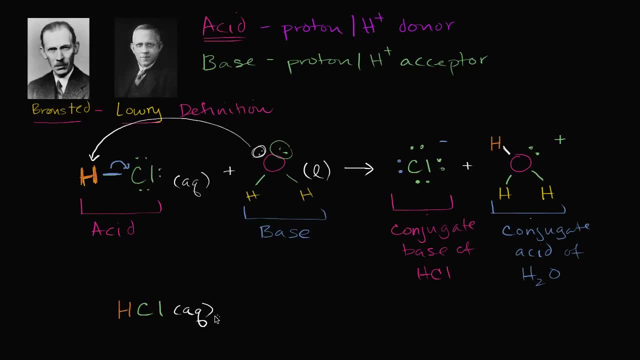 in an aqueous solution, So it's in a solution of water, And they'll just draw the reaction going like this where they say, hey, you're going to be left with, you're going to be left with some hydrogen ions.